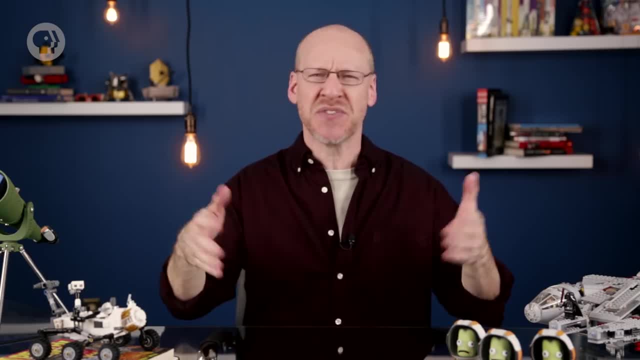 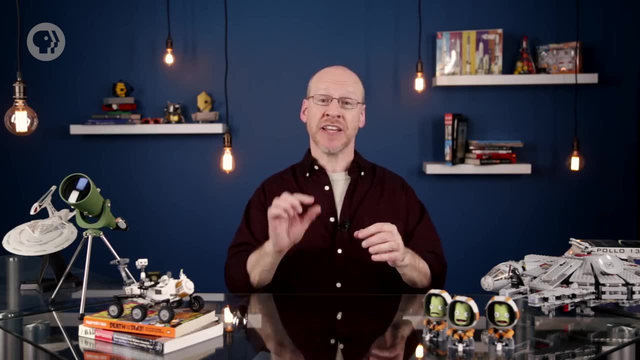 so he could find the distance between them, But more likely, he just used the numbers found by earlier surveying missions. Either way, knowing the distance and the angle and applying a little geometry, he calculated the circumference of the Earth. His result, a little over 40,000 kilometers, is actually. 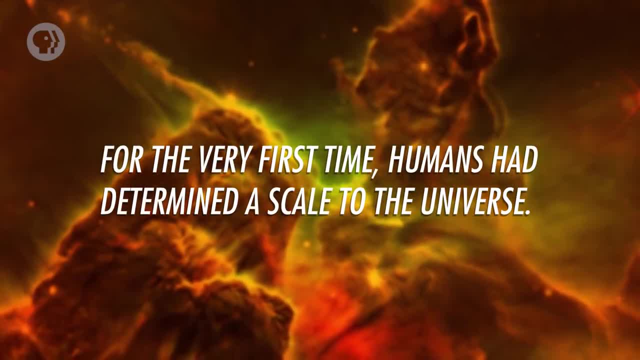 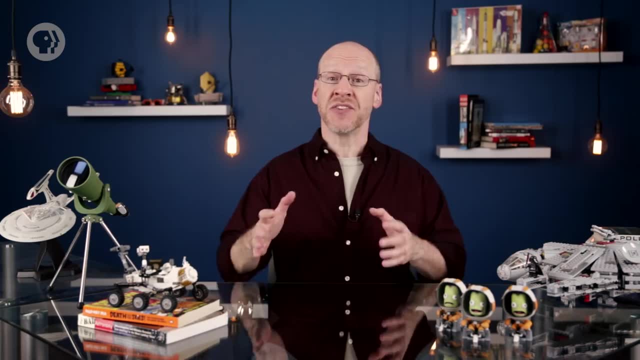 amazingly accurate. For the very first time, humans had determined a scale to the Universe. That first step has since led to a much, much longer journey. Once you know how big the Earth is, other distances can be found, For example, when 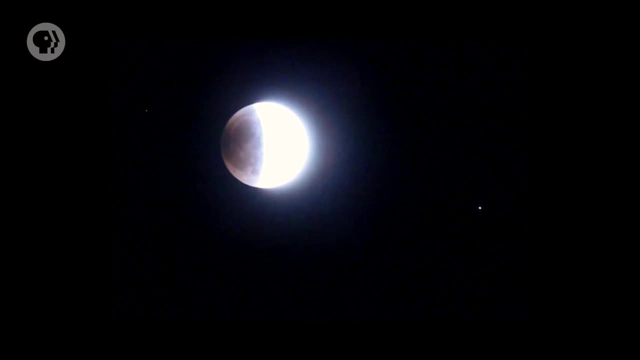 there's a lunar eclipse, the shadow of the Earth is cast on the Moon. You can see the curve of the Earth's edge at the end of the Earth. It's a very long, long, long, long, long edge as the shadow moves across the Moon. Knowing how big the Earth is and doing 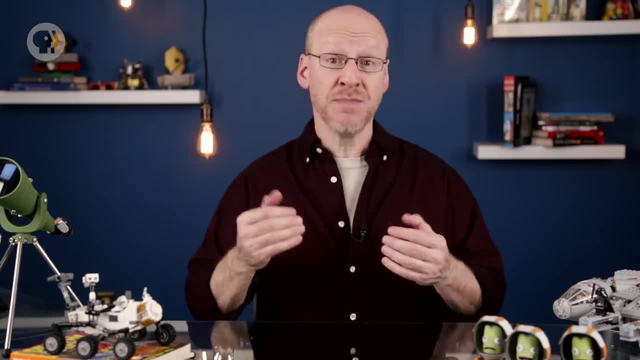 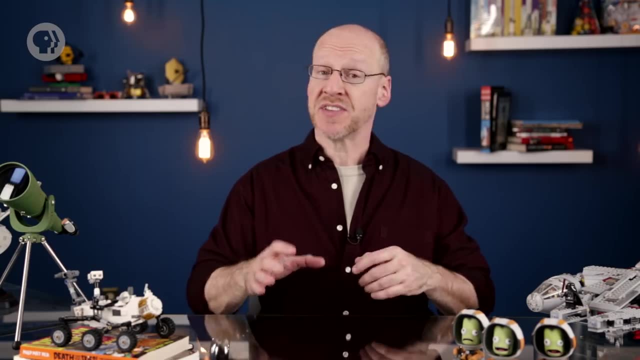 a little more geometry, you can figure out how far away the Moon is. Also, the phases of the Moon depend on the angles and distances between the Earth, Moon and Sun. Using the size of the Earth as a stepping stone, Aristarchus of Samos was able. 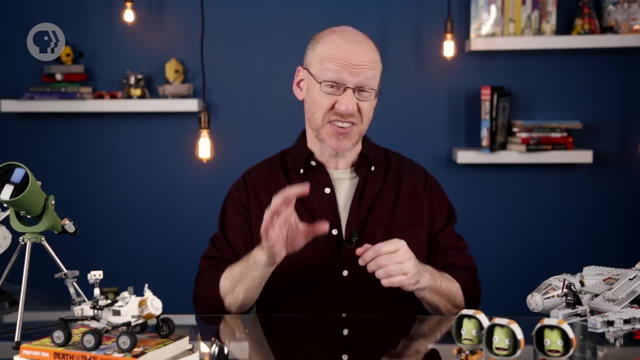 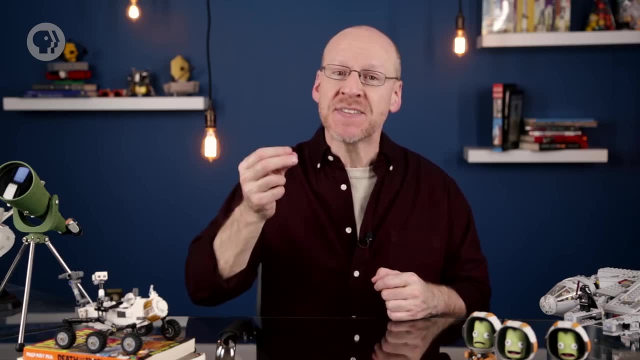 to calculate the distances to the Moon and the Sun, as well as their sizes. That was 2,200 years ago. His numbers weren't terribly accurate, but that's not the important part. His methods were sound and they were used to calculate the distance between the Earth and the Sun. 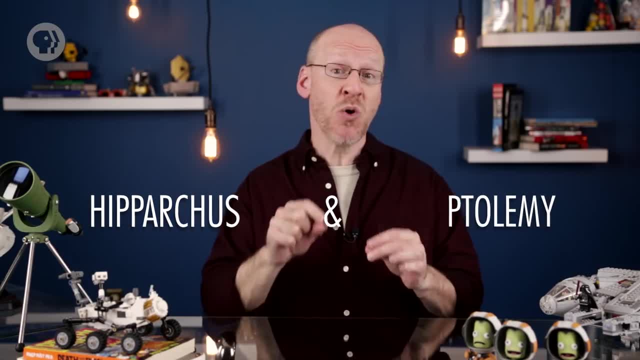 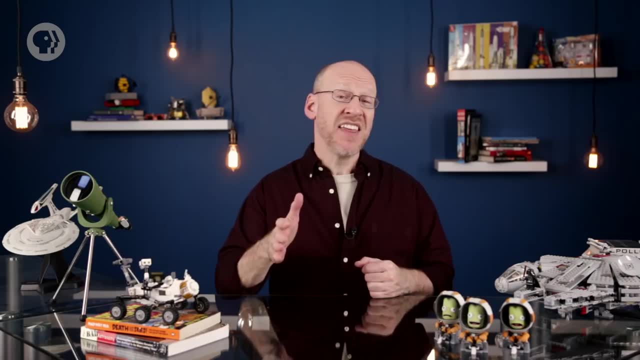 and they were used later by great thinkers like Hipparchus and Ptolemy to get more accurate sizes and distances. They actually did pretty well, and all over a thousand years before the invention of the telescope, And I think it also says a lot that these ancient thinkers were willing to accept a 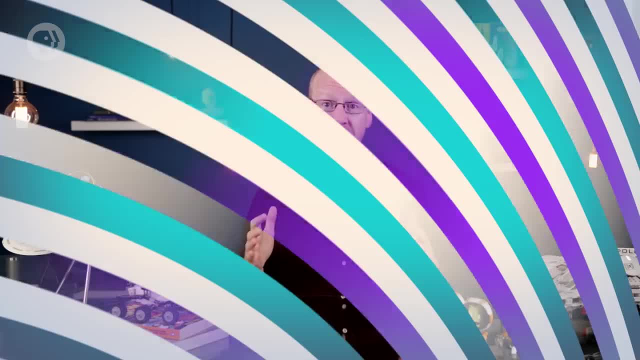 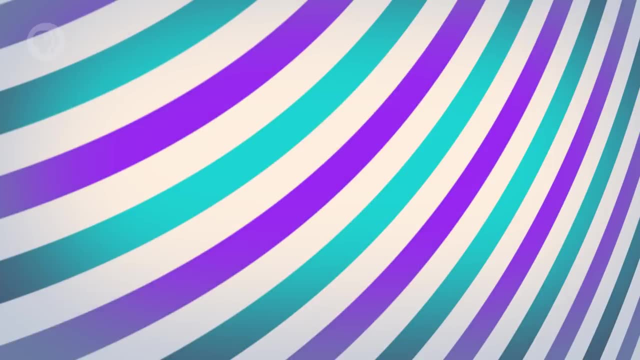 solar system that was at least millions of kilometers in size. But at this point things got sticky. Planets are pretty far away and look like dots. Our methods for finding distances failed for them For a while at least, In the 17th century. 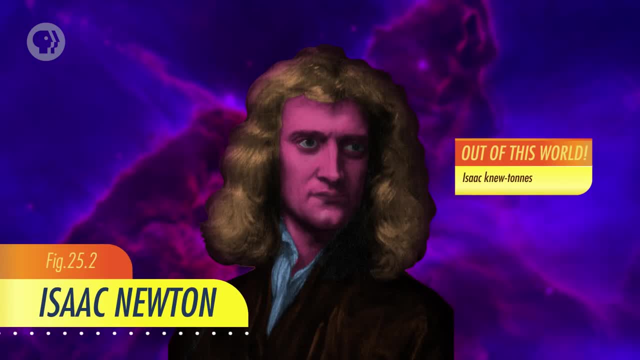 Johannes Kepler and Isaac Newton laid the mathematical framework for finding distances, and they were able to do it, They were able to do it, and they were able to do it, and they were able to do it. They laid the mathematical groundwork of planetary orbits and that. 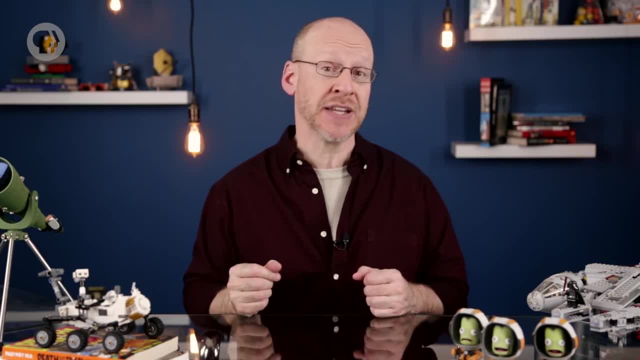 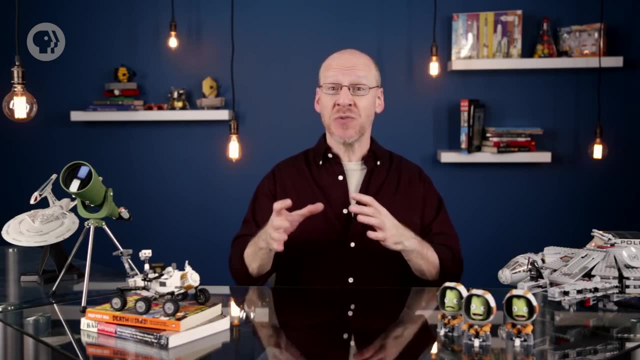 in turn, made it possible in theory to get the distances to the planets. Nah, but there was a catch. When you do the math, you find that measuring the distances to the other planets means you need to know the distance from the Earth to the Sun accurately. 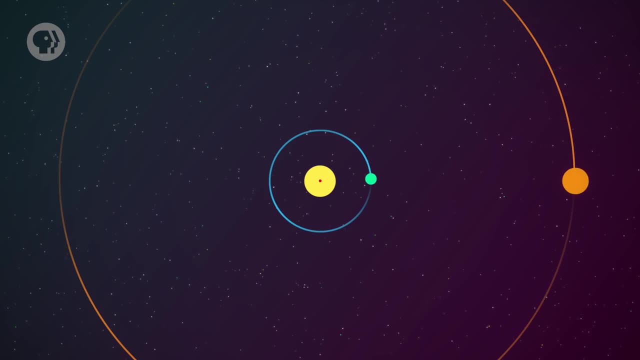 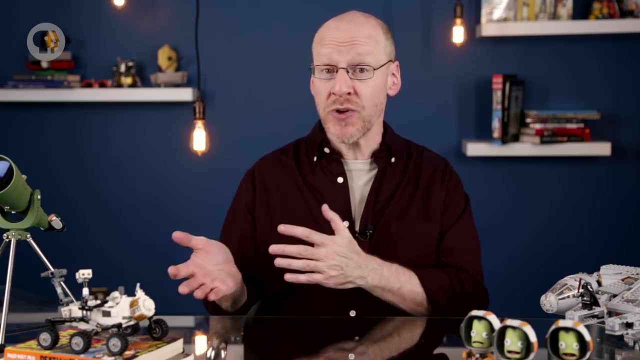 For example, it was known that Jupiter was about five times farther from the Sun than the Earth was, But that doesn't tell you what it is in kilometers. So how far away is the Sun? Well, they had a rough idea using the number found by the Greeks. but to be able to truly 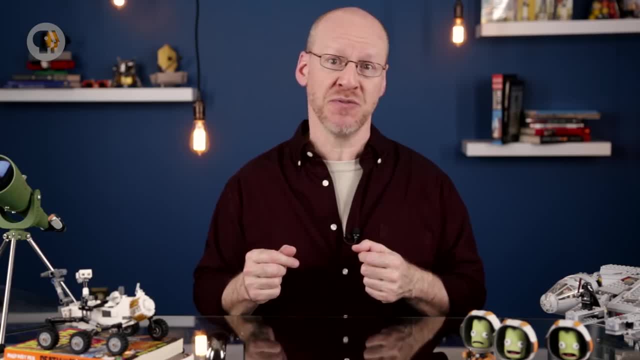 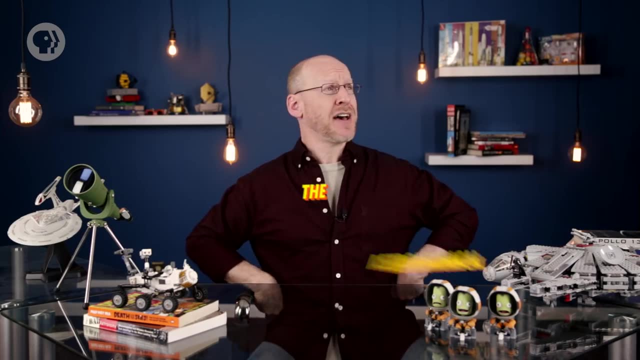 understand the solar system, they needed a much more accurate value for it. To give you an idea of how important the distance from the Earth to the Sun is, they gave it a pretty highfalutin name: the Astronomical Unit or AU, Mind you, not an astronomical. 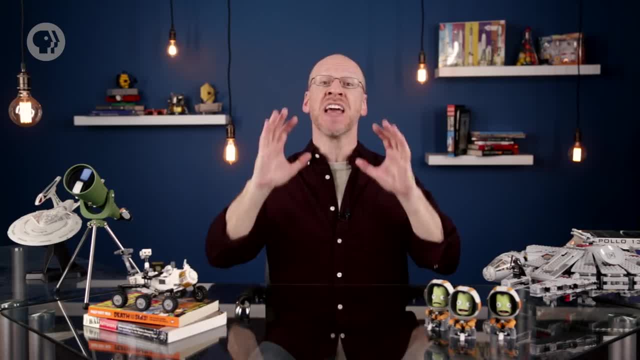 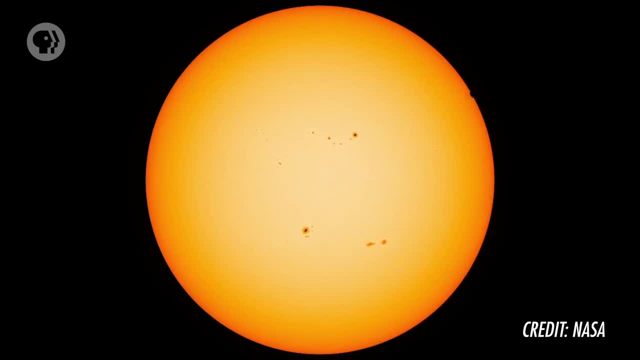 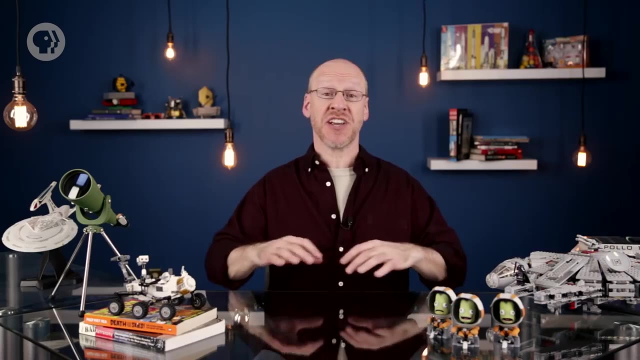 unit the one. That's how fundamental it is to understanding everything. A lot of methods were attempted. Sometimes Mercury and Venus transit or cross the face of the Sun. Timing these events accurately could then be used to plug numbers into the orbital equations and get the length of an AU. Grand expeditions were sent across the 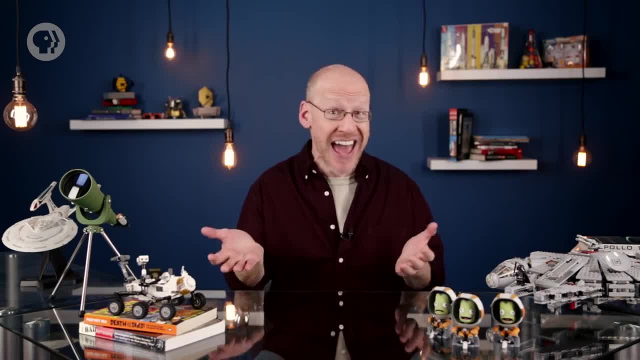 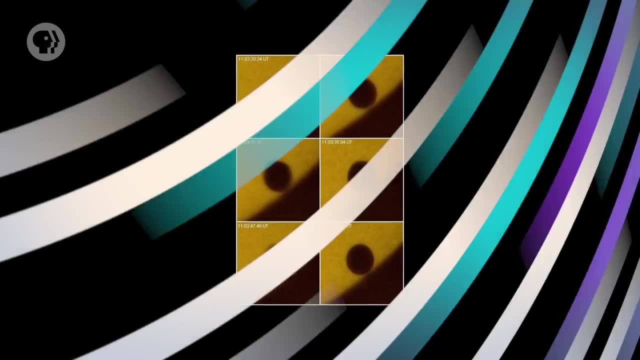 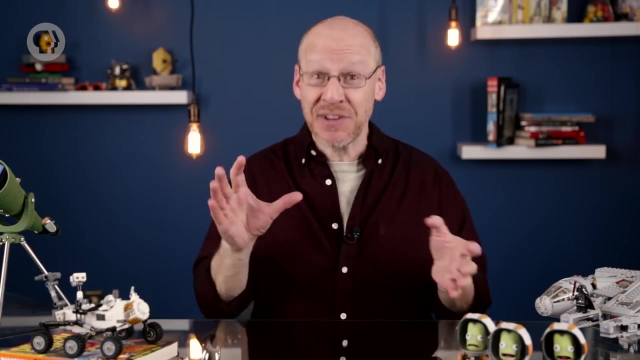 globe multiple times to measure the transits and didn't do too badly. But our atmosphere blurs the images of the planets, putting pretty big error bars on the timing measurements. The best they could do was to say the AU was 148,510,000 kilometers plus or minus 800,000. 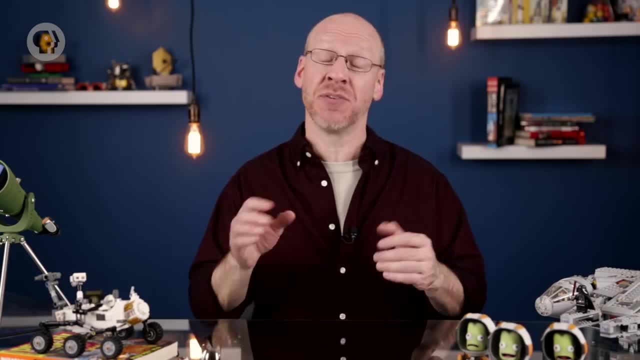 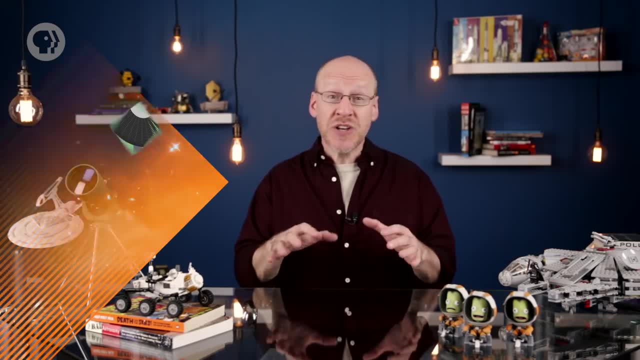 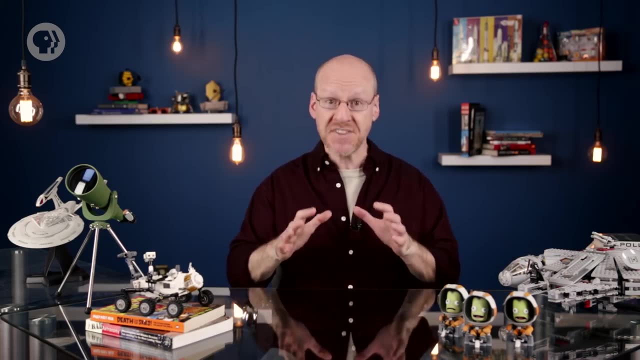 to measure the transits. They used radio telescopes to bounce radar pulses off of Venus. Since we know the speed of light extremely accurately, the amount of time it takes for the light to get to Venus and back could be measured with amazing precision. 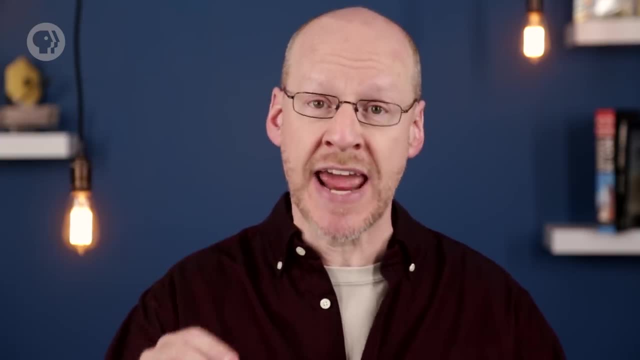 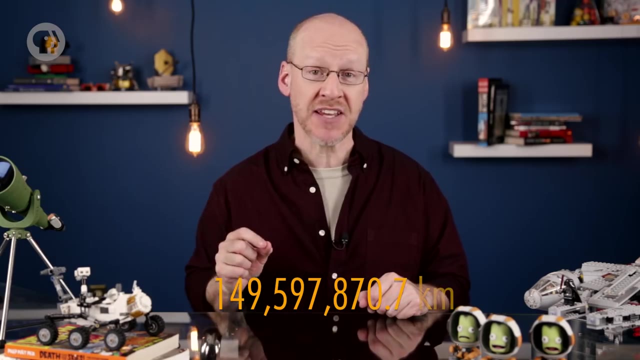 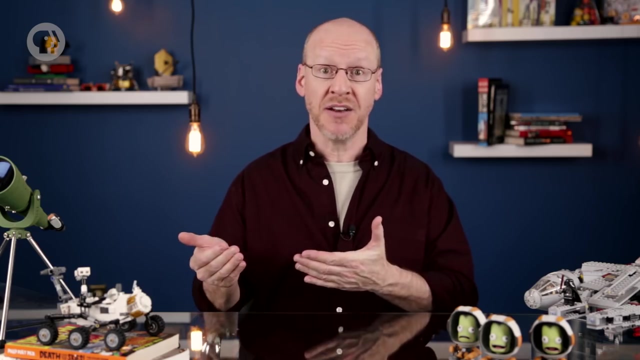 Finally, after all these centuries, the astronomical unit was nailed down. It's now defined to be 149,597,870.7 kilometers. So there, The Earth orbits the Sun on an ellipse. so think of that as the average distance of the Earth from the Sun. Knowing this number, we can't 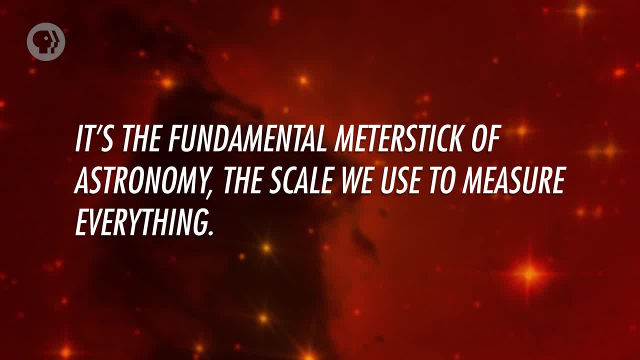 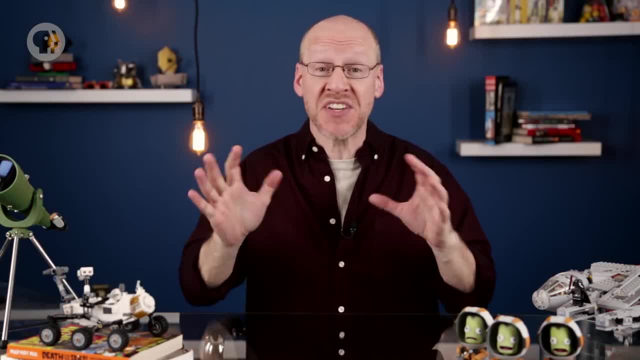 predict how far it will go. But knowing this number unlocked the solar system. It's the fundamental meter stick of astronomy and the scale we use to measure everything. Having this number meant we could predict the motions of the planets, moons, comets and asteroids. Plus, it meant we could. 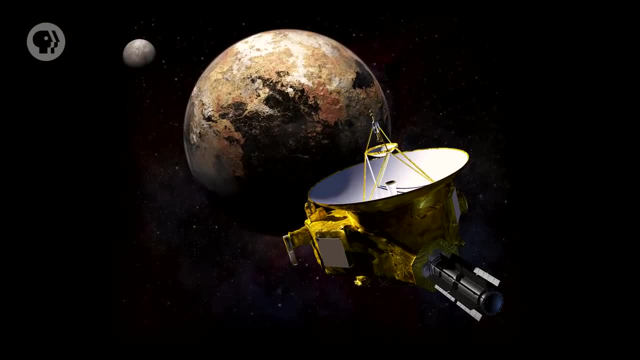 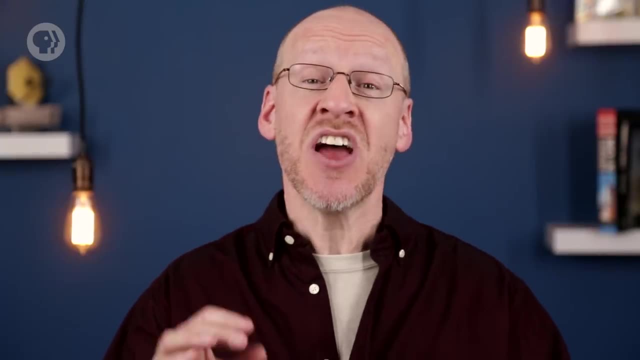 launch our probes into space and explore these strange new worlds for ourselves, see them up close and truly understand the nature of the solar system. And it's even better than that. Knowing the astronomical unit meant unlocking the stars. We have two eyes and 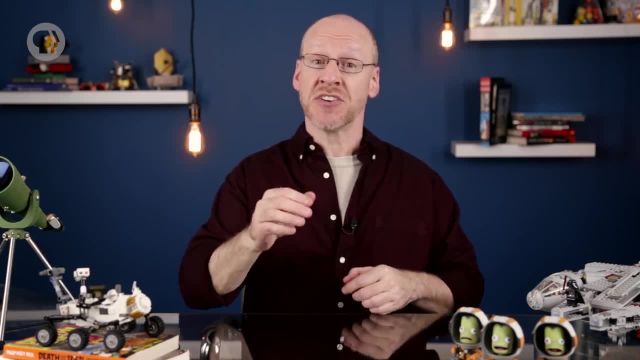 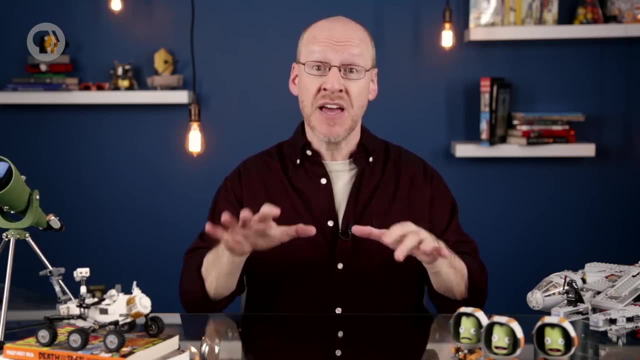 this gives us binocular vision. When you look at a nearby object, your left eye sees it at a slightly different angle than your right eye. Your brain puts these two images together, compares them, does the geometry, and gives you a sense of distance to that object. 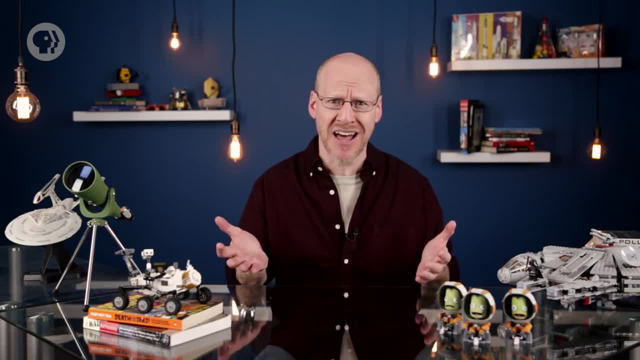 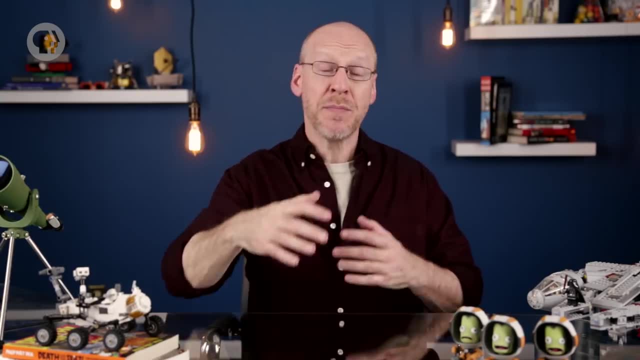 And you thought your teacher lied when she said math was useful in everyday life. We call this ability depth perception. You can see it for yourself by doing the thumb thing. As you blink one eye and then the other, your thumb appears to shift position relative. 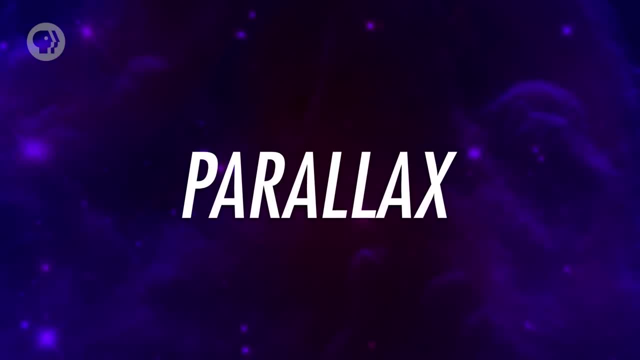 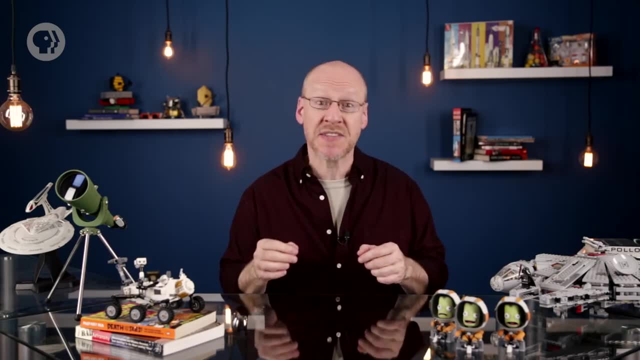 to more distant objects. That shift is called parallax. The amount of shift depends on how far apart your eyes are and how far away the object is. If you know the distance between your eyes- we'll call this the baseline- then you can apply some trigonometry and figure out how far away the object is. If the object 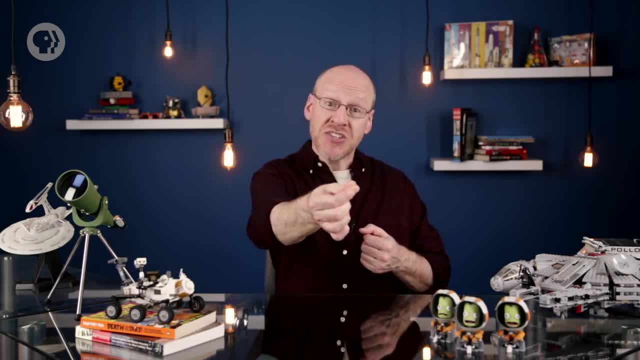 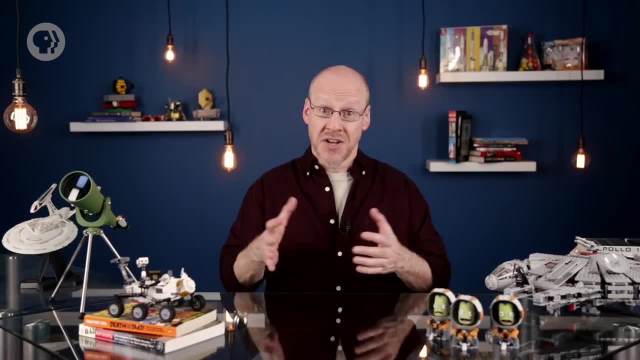 is nearby, it shifts a lot. If it's farther away, it shifts less. It works pretty well, but it does put a limit on how far away we can reasonably sense distance with just our eyes. Stars are a bit beyond that limit If we want to measure their distance using parallax. 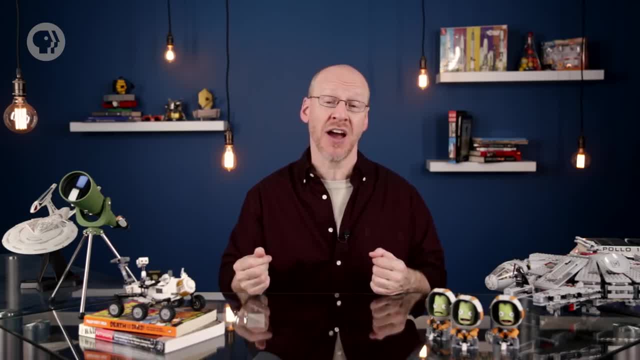 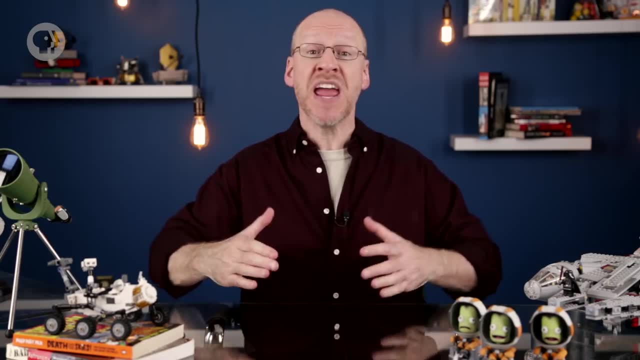 we need a lot bigger baseline. Once astronomers figured out that the Earth went around the Sun rather than vice versa, they realized that the Earth's orbit made a huge baseline. If we observe a star when the Earth is at one spot, then wait six months for the Earth. 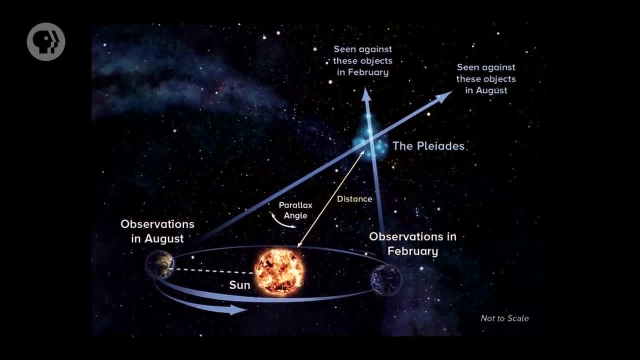 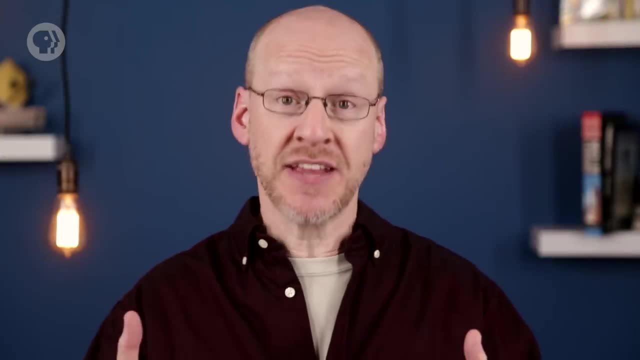 to go around the Sun to the opposite side of its orbit and observe the star again. then in principle we can determine the distance to the star, assuming we know the size of the Earth's orbit. That's why knowing the length of the astronomical unit is so important. The diameter of Earth's 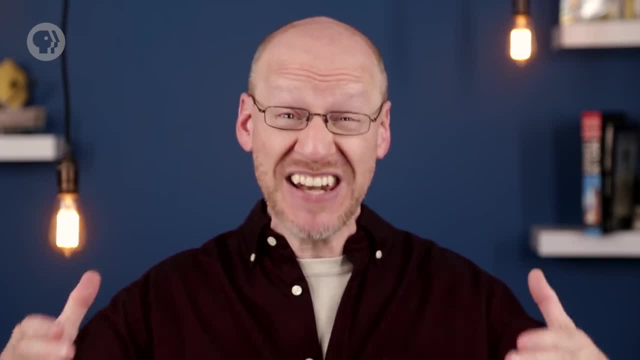 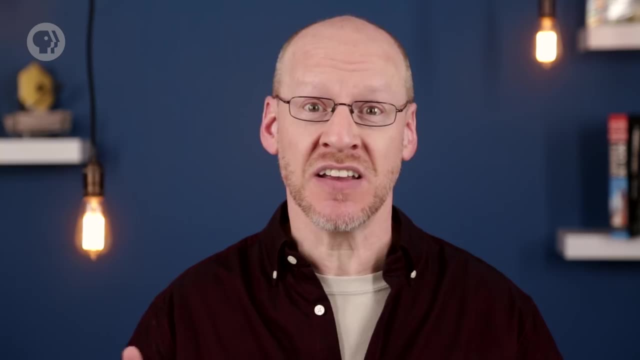 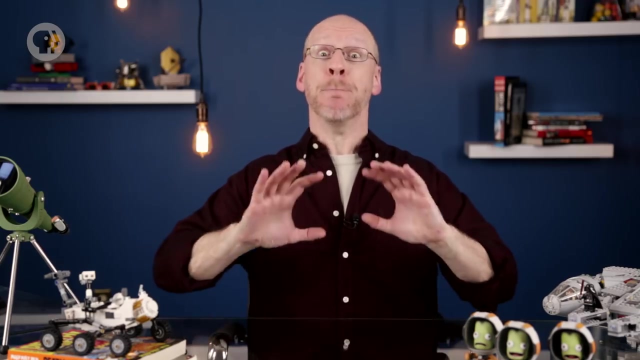 orbit is about 300 million kilometers, which makes for a tremendous baseline. Hooray, Exceptoops. When stars were observed, no parallax was seen. Was heliocentrism wrong? Pfft, No, It's just that stars are really and truly far away, much farther than even. 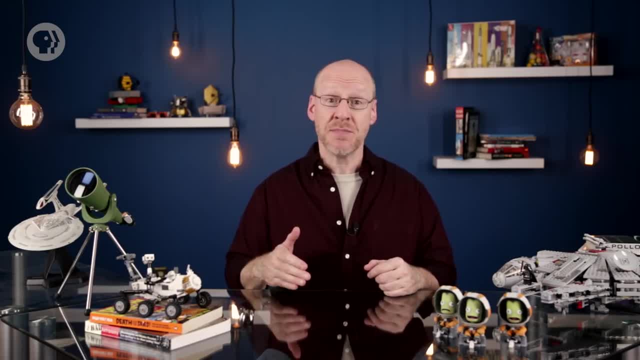 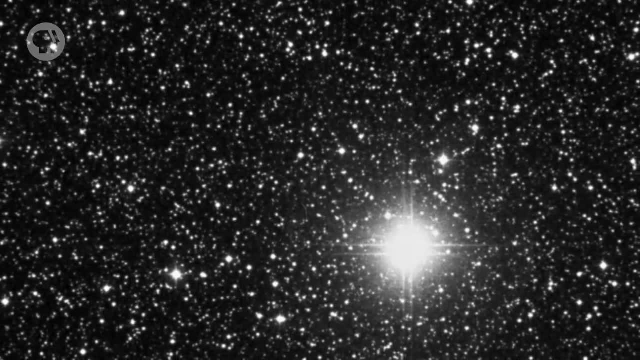 the size of Earth's orbit. The first star to have its parallax successfully measured was in 1838.. The star was 61 Cygni, a bit of a dim bulb, but it was bright enough and close enough astronomers to measure its shift in apparent position as the Earth orbited the Sun. 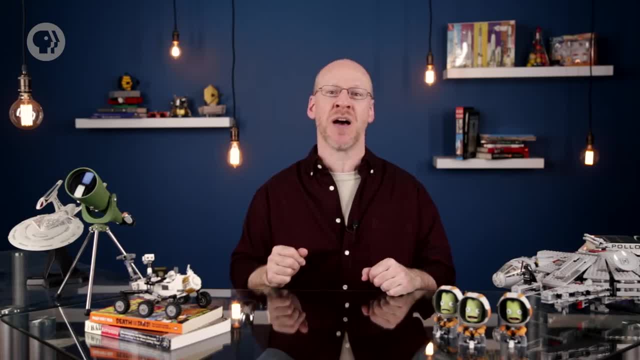 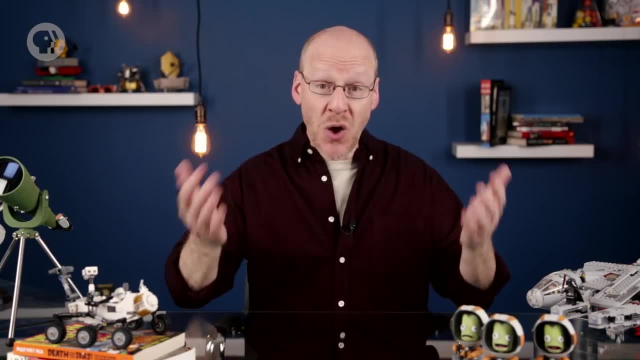 61. Cygni is about 720,000 astronomical units away. That's a soul-crushing distance, well over 100 trillion kilometers. In fact, that's so far that even the Earth's orbit is too small to be a convenient unit. 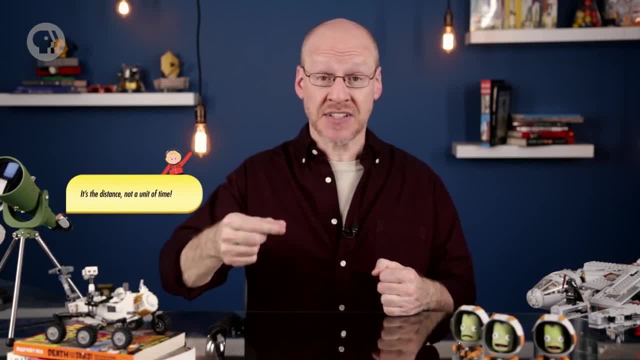 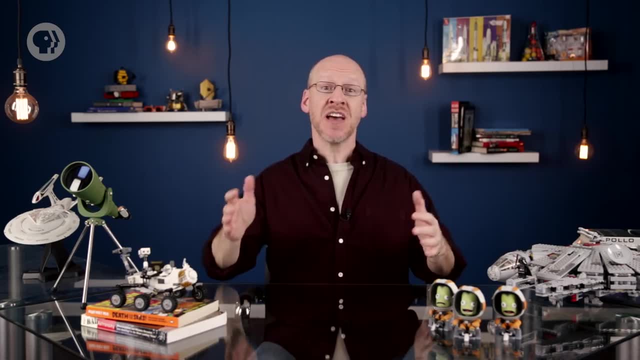 Astronomers came up with another one: the light year. That's the distance light travels in a year. Light's pretty fast and covers about 10 trillion kilometers in a year. It's a huge distance, but it makes the numbers easier on our poor ape brains. 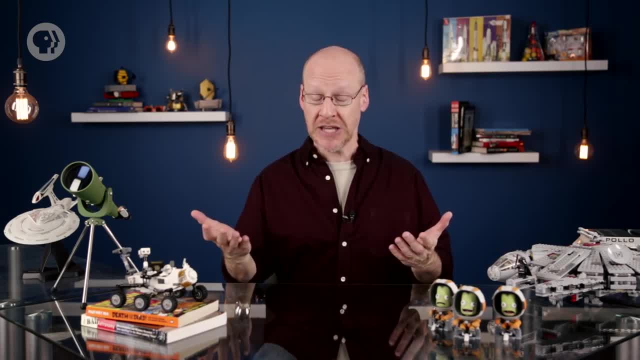 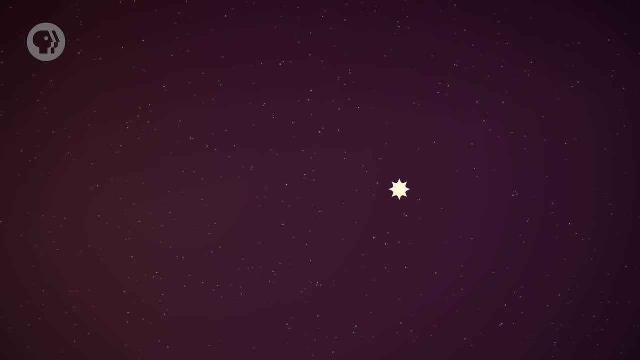 That makes 61 Cygni a much more palatable, 11.4 light years away. Astronomers also use another unit called a parsec. It's based on the angle a star shifts over the course of a year. A star one parsec away will have a parallax shift of. 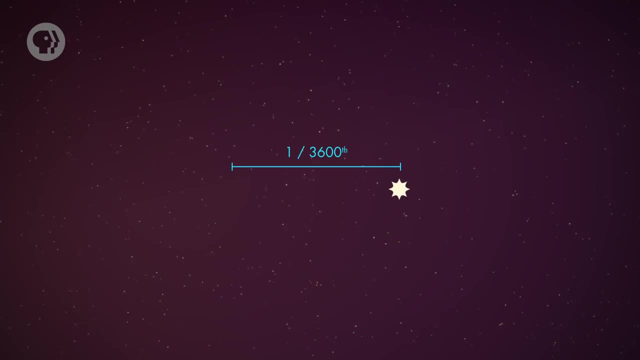 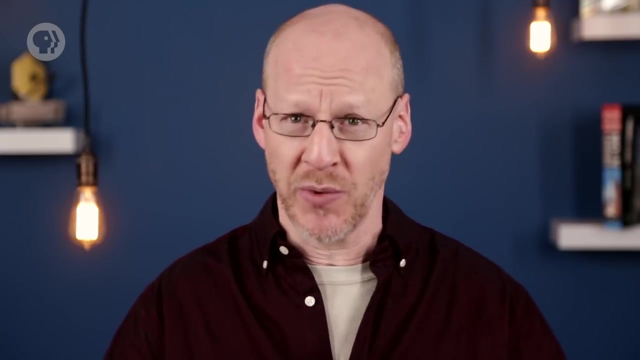 one arc second, 1, 36 hundredth of a degree. That distance turns out to be about 3.26 light years. As a unit of distance, it's convenient for astronomers, but it's a terrible one if you're doing the Kesselman. Sorry, Han. The nearest star to the Sun we know of, Proxima Centauri, is about 4.2 light years away. The farthest stars you can see with the naked eye are over a thousand light years distant, but the vast majority are within 100 light years. 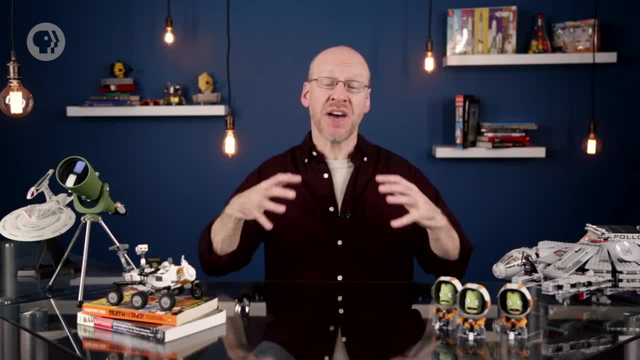 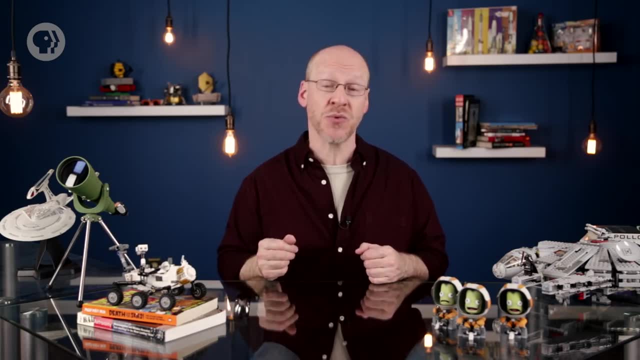 Space-based satellites are used now to accurately find the distance to hundreds of thousands of stars. Still, this method only works for relatively nearby stars, ones that are less than about a thousand light years away. But once we know those distances, we can use that. 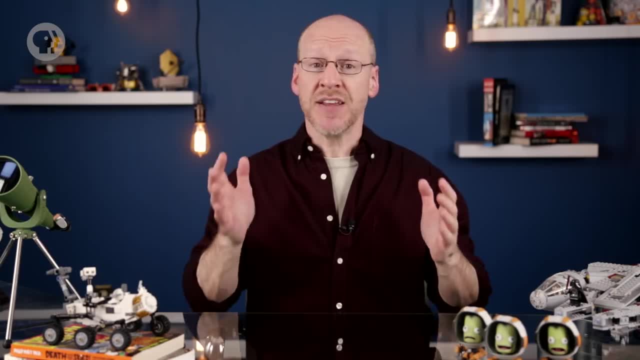 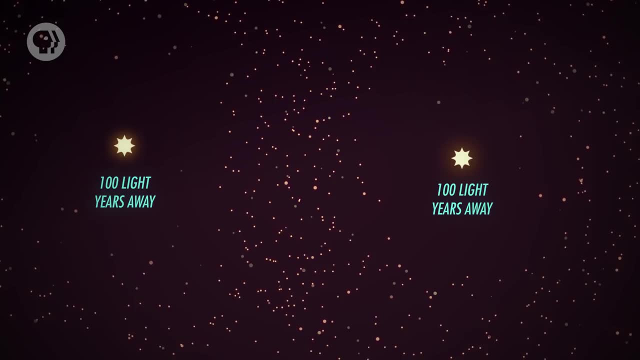 information on more distant stars. How Basically the strength of light falls off with the square of the distance. If you have two stars that are the same intrinsic brightness, giving off the same amount of energy, and one is twice as far as the other, it will be one quarter as bright. Make it ten times. 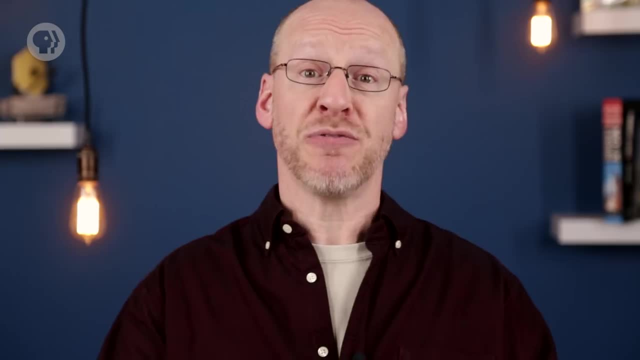 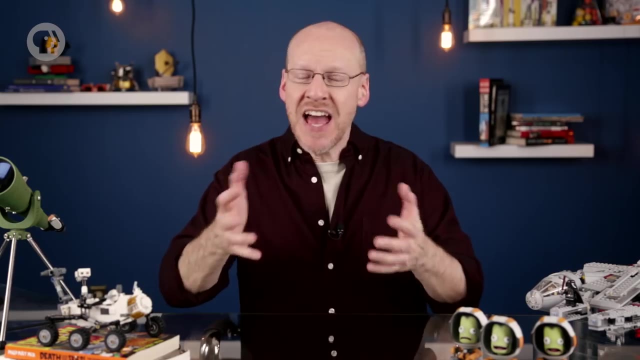 farther away it'll be one one hundredth as bright. So if you know how far away the nearer one is by measuring its parallax, you just have to compare its brightness to one farther away to get its distance. You have to make sure they're the same kind of star. Some are more luminous than others. 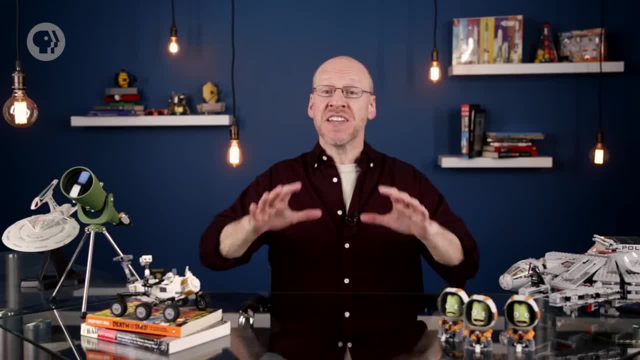 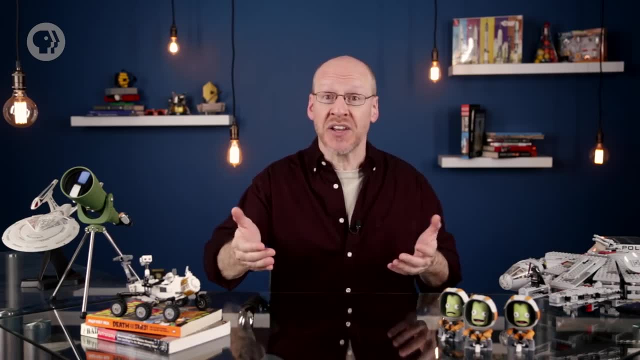 But thanks to spectroscopy we can do just that. Stars' distance is the key to nearly everything about it. Once we know how far it is and we can measure its apparent brightness, we can figure out how luminous it is, how much. 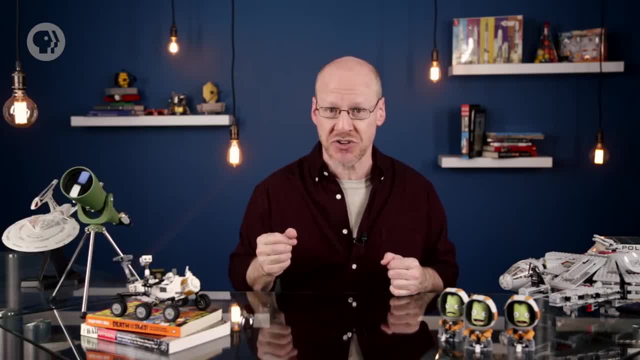 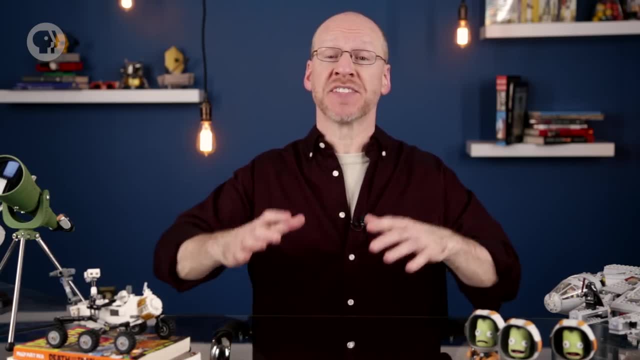 light it's actually giving off and its spectrum tells us its temperature. With those in hand, we can determine its mass and even its diameter. Once we figured out how far away stars are, we started to grasp their true physical nature. This led to even more methods of finding distances: The light given off by dying stars exploding.